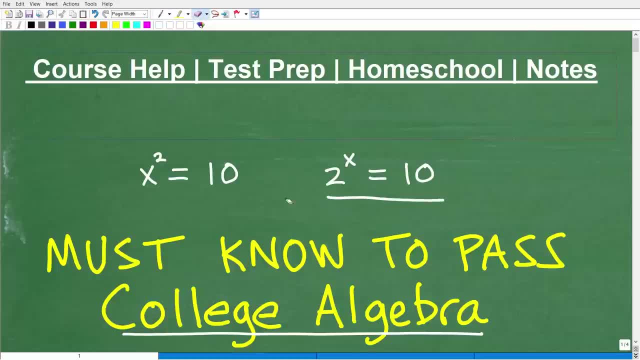 This problem. although they might look a little similar, what we do is completely different. So this is definitely college algebra level stuff, or algebra two at the high school level. So if you're at the, you know, taking any sort of algebra course, okay, you want to stick around, because it doesn't have to be just college algebra. You can be taking an intermediate algebra course or some other type of course that has algebra. Now this is going to apply to you as well. So we're going to get into all of this in just one second. But 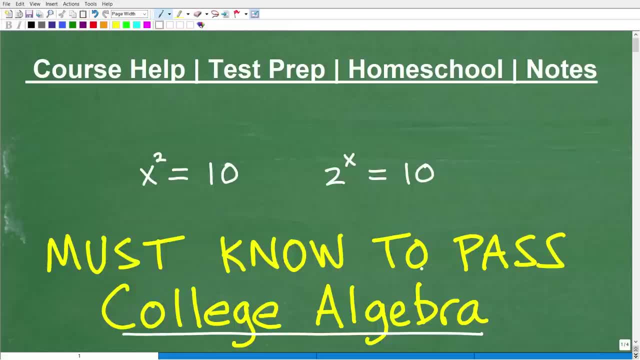 first, let me quickly introduce myself. My name is john. I'm the founder of tablet class math. I'm also a middle and high school math teacher. I'm going to leave a link to my math help program in the description of this video, But if you are having a difficult time in math, I'm here to tell you. it doesn't have to be that way. Okay, so I have not met any bad math students over decades of teaching mathematics. Okay, if you have the desire to want to learn. okay, if you're willing to work right, you. 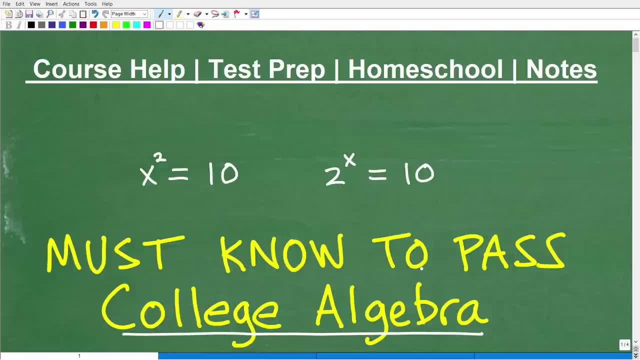 can be successful. So when I talk about you know, if you think you're a bad math student, that just means that you're not. you haven't found success. But you can find success, which you need. okay, if you're willing to put into work and do all the you know your part. what you need is the right instruction. So that's very clear and understandable. So that's my teaching style. Okay, I really like to explain things in super easy, bite sized pieces so that any student, every student, can learn this stuff. Okay. so if you're at the middle school, high school or college level, I 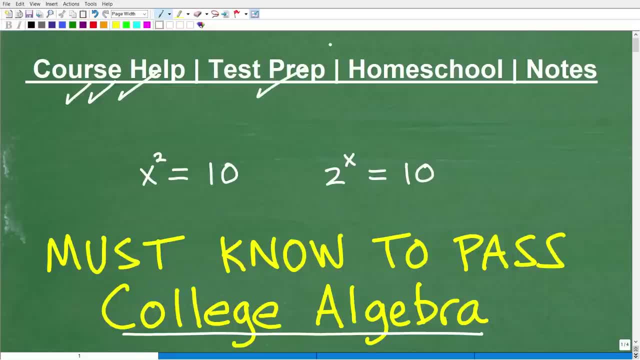 can definitely help you out. Now, if you happen to be preparing for any test that has a math section on it- I'm talking about things like the GED, SAT, ACT, GRE, GMAT, ASVAB, ACCUPLACER, CLIP exam, maybe a teacher certification exam- I can definitely help you prepare and pass those exams. If you homeschool well, you definitely have to check out my homeschool math courses. we were just voted number one in middle and high school mathematics by a pretty major homeschool publication. 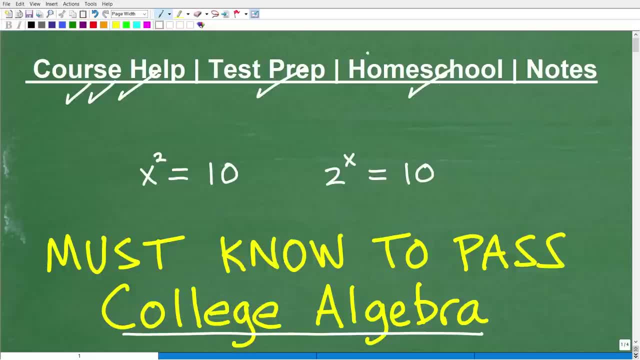 and we're pretty proud of that. we're going to be announcing more about that, So definitely check out our homeschool math courses And if you need some math notes, I'm going to leave links to my math notes also in the description of this video. But if you want great grades in math, you must learn how to take great math notes. So start improving your notes and everything will start getting better. Okay, so let's get into these two equations. They look similar, okay, but they are quite different. Of course, I'm going to solve. 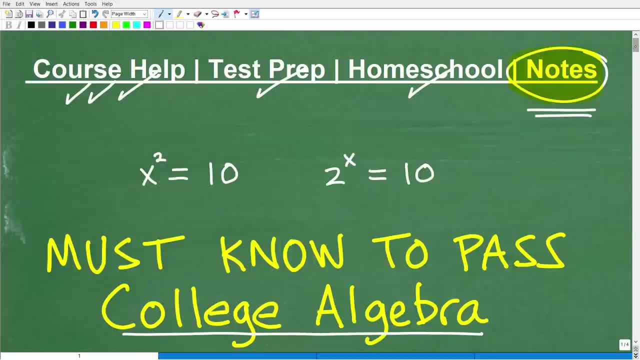 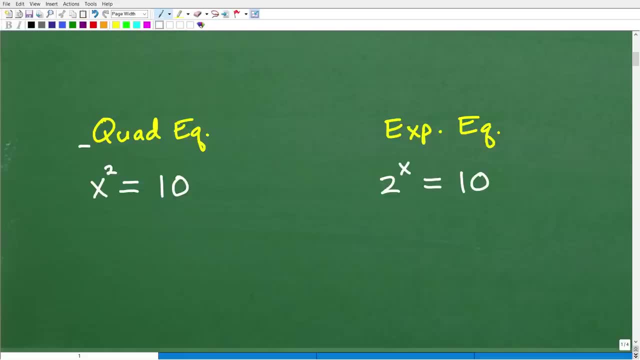 both of these here in a second, But let's go down and take a look at what's going on here, Okay, Well, first thing is this: right before you do anything, you need to be able to identify what type of equations we're dealing with here. So this first equation: x squared is equal to 10, is a what? Well, hopefully you recognize that as a quadratic equation. So this is the kind of stuff you study like an algebra one. So what can you tell me about quadratic equations? Okay, I'm just 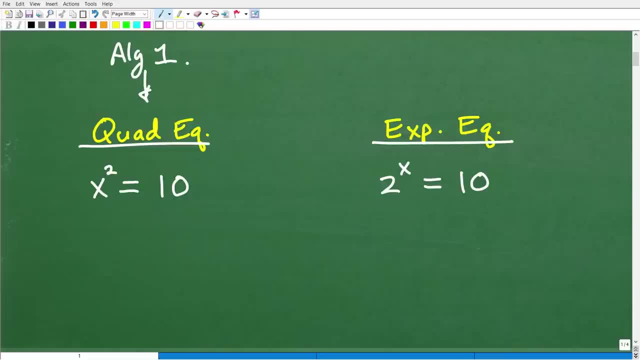 asking you, So put some of your answers into the comment section. How do we solve quadratic equations? Okay, so that's a question for you. The second thing is: how many solutions does a quadratic equation have? All right, so let's go ahead and just answer this right now. So quadratic equations will always have two solutions, always, always. 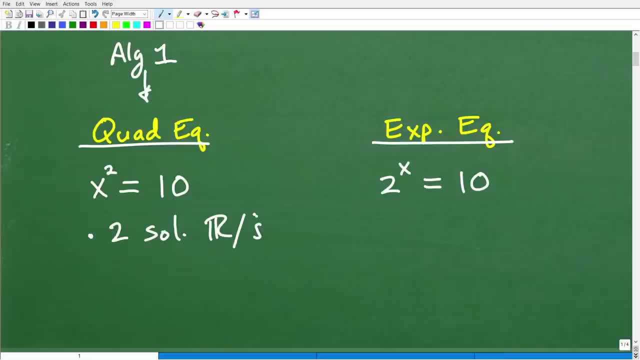 sometimes they're going to be real number solutions or imaginary number solutions, but they're always going to have two solutions. Now, how we solve quadratic equations? well, there's all kinds of different techniques, and this is stuff, again, you should have mastered in algebra- one- you probably are reviewing this already, like in: 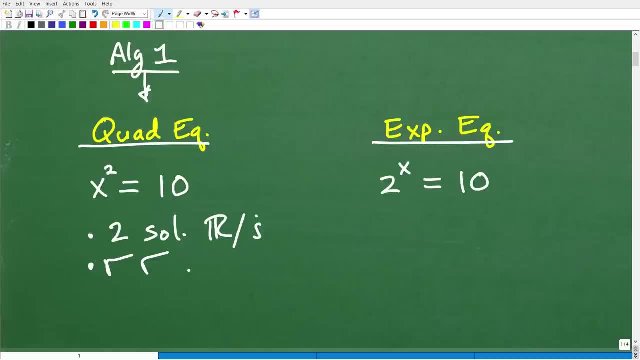 the college algebra course. but sometimes you can take the square root of both sides, sometimes you can factor, sometimes you have to use the quadratic formula, then there's something called completing the square. so there's quite a bit of different techniques involved in solving quadratic equations. okay, so these are some just right. here is just some basic overviews of quadratic equations. so 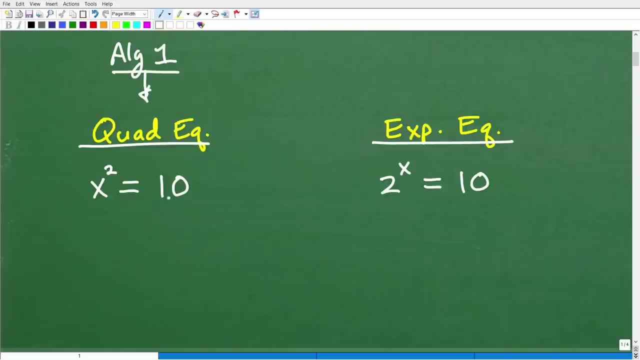 let's go ahead and solve this. and we have: x squared is equal to 10. so the easiest way to solve this is simply to take the square root of both sides. so the square root of x squared is x and the square root of 10. now, here we're not talking about the principal square root. 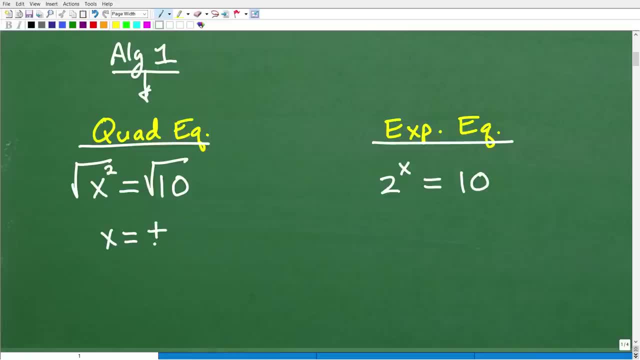 we're going to be talking about the plus and minus version, so the square root of 10 is plus and minus the square root of 10. okay, so, for example, if I took the square root of 4, the answer is going to be plus or minus 2. why? because positive. 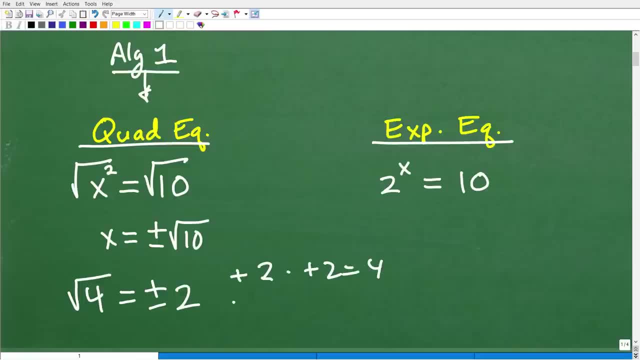 2 times positive 2 is positive 4 and negative. 2 times negative 2 is also a positive 4. so these are our two solutions here, both positive and negative. okay, remember, quadratic equations have two solutions. so over here, okay, our two solutions would be what? well, one solution is. 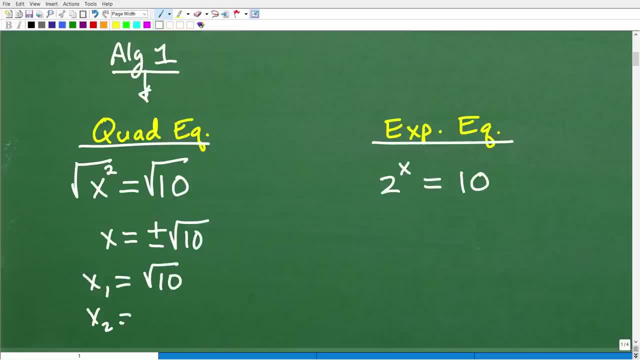 going to be positive square root of 10, and our second solution is negative square root of 10. so instead of writing this way- positive square root of 10, negative square root of 10- it's pretty, um pretty common just to write this notation plus or minus right here. it just saves us, uh, for having us to write these two unique. 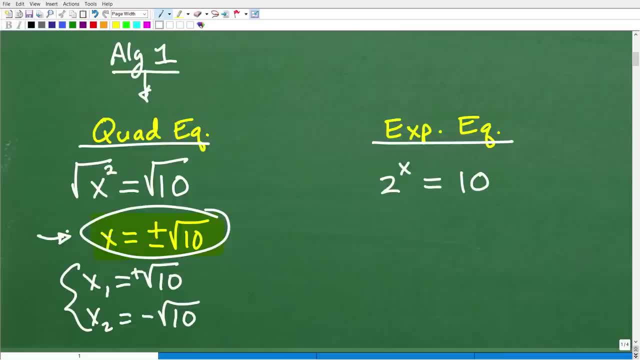 solutions, but just remember, there are two unique solutions to this quadratic equation. all right, so if you got that right, that's excellent and give you a little check mark here. so now let's talk about this equation. okay, so what are we talking about here? you can see, I have it a. 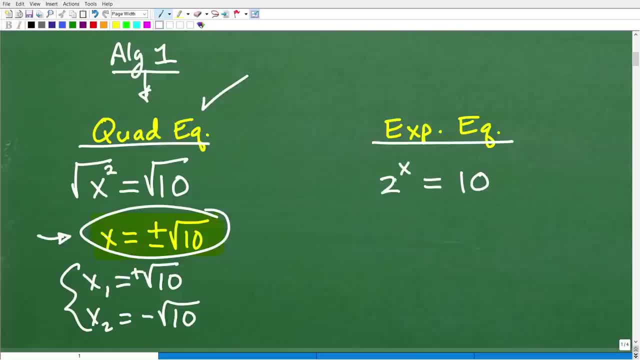 little abbreviated. well, uh, this, uh. in this particular equation the variable is an exponent. okay, so down here, this uh. x was down in the base, all right, and we recognize this as a polynomial to degree two, but here the variable that we're looking for is in the exponent. so we would classify: 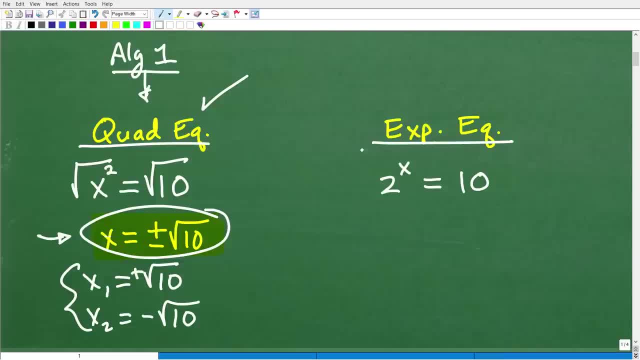 this as an exponential equation, because this is an exponential equation. if you knew that, that's excellent. so how do we solve exponential equations? okay, well, you need to use something called logarithms. okay, so, when we see an exponential equation, we're going to have to use logarithms to solve it. when we see a logarithmic equation, we're going to have to use 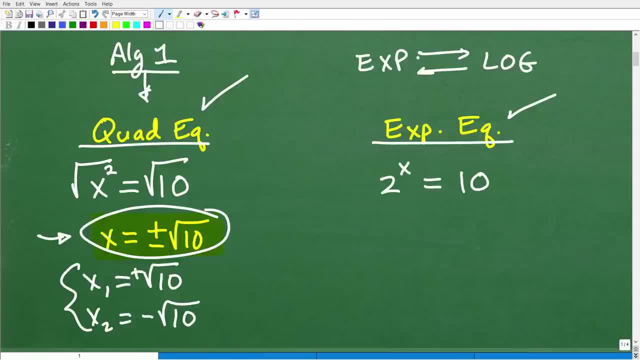 exponents to solve logarithmic equations, because exponential functions and logarithmic functions are inverse functions of one another. okay, so you're going to have to know both of these when you're at that college algebra, algebra 2 level. okay, so I kind of gave you some hints here. 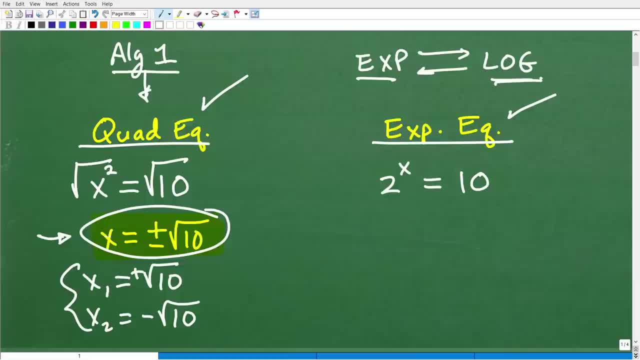 all right, uh, this is, this is an exponential equation and you're going to be using logarithms to solve. so just in case you forgot that and you're like, okay, now I remember that, well then, let me go ahead and see, do this problem, go ahead and pause the video and solve for x. okay, so we know how to do this. 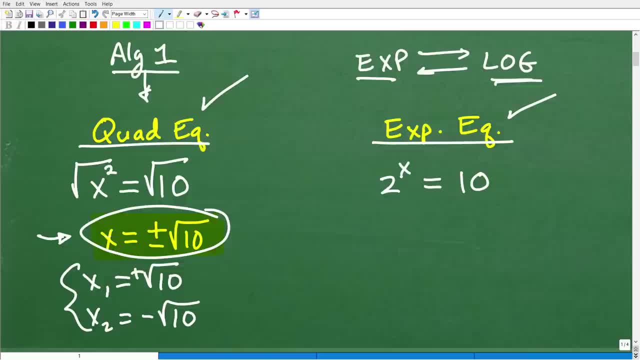 this will take you about 30 seconds, but I'm going to go ahead and do this now. all right, so the first thing we want to do is just take the log of both sides, the logarithms of both sides, and we'll go. log 2 x is equal to log 10.. 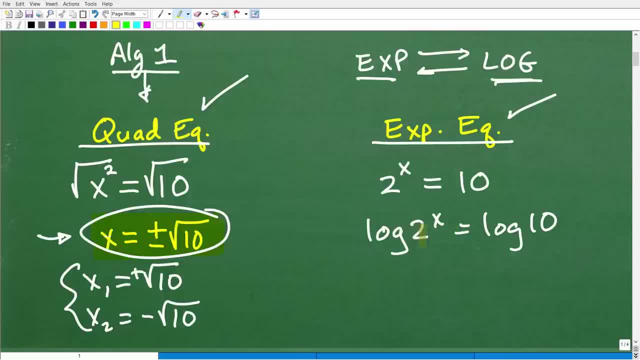 if you go to your calculator, okay, you put in log 2, log2, you'll see that this is just a number itself. log10 is just number in and of itself. so these are just numbers, okay. so let me just uh write this right, make this uh much clearer. okay, so I'm taking the log of both sides. now I want to solve for x, so 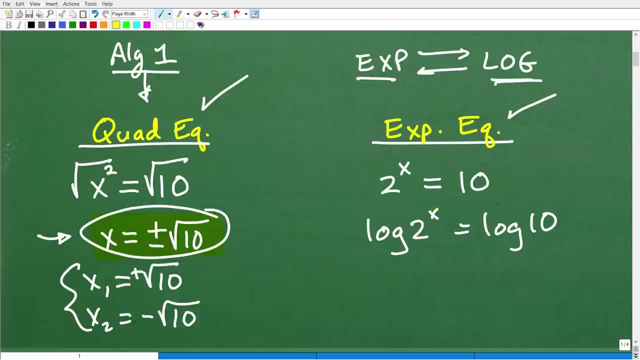 what we need to now know is a property of logarithms. so I have a problem. I don't have personally the property. there is a problem that says that we can drop this variable, this little exponent in front of the log. this is how we unlock this solution, so I'm going to take this X and rewrite it. 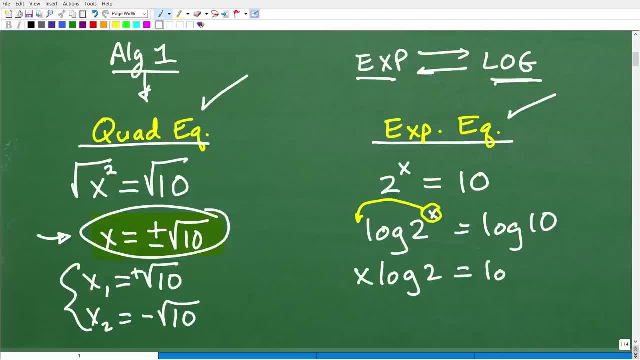 down here. X log 2 is equal to log 10. okay, all right. now again, by using my calculator, log 2 is just a decimal. I can find on my calculator same thing with log 10. okay, this is called the common logarithm. I'm skipping a lot of stuff. 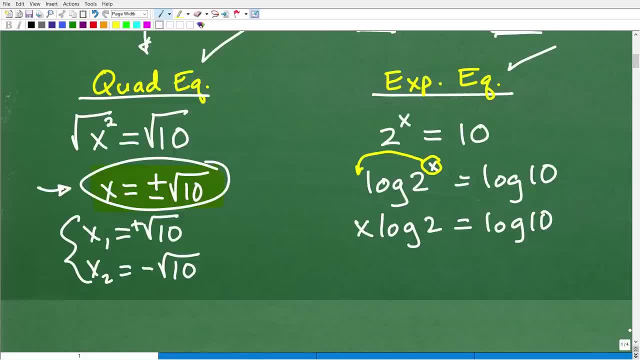 here I'm not really talking about what a logarithm is, etc. but really what you need to know is logarithms are powerful, they allow us to solve exponential equations and you'll need your calculator for most problems. okay, so we have X times a number. okay, that this. again, this is a decimal, so X times some. 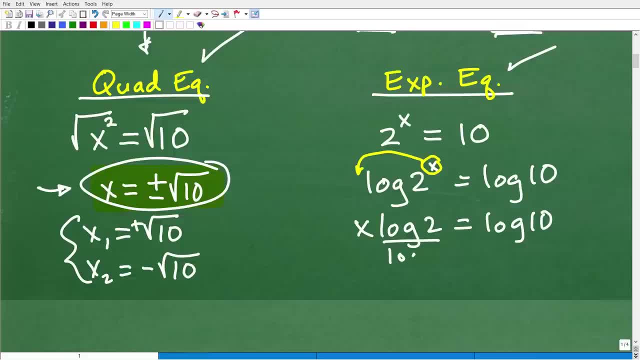 number is equal to another number. so how do I solve for X? well, I just simply divide both sides of the equation by log 2, and so X is going to be equal to log 10 divided by log 2. of course I can go into my calculator and get. 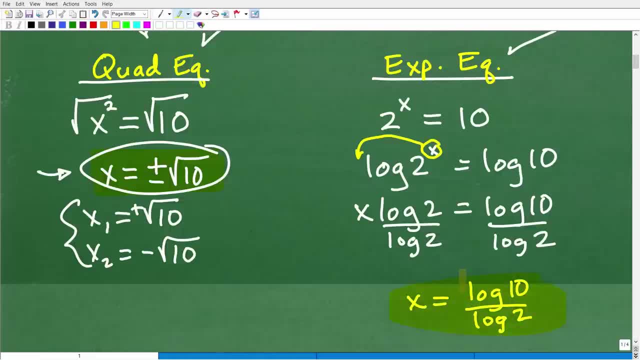 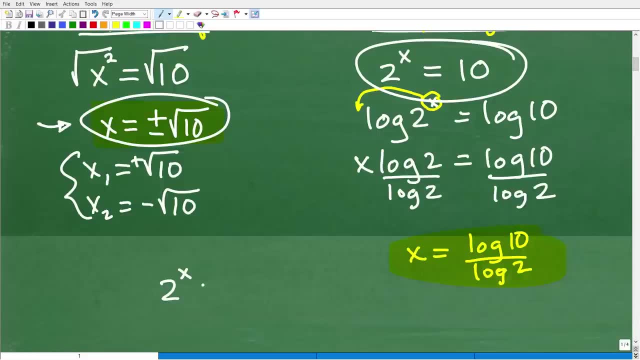 that actual decimal and you'll get the right answer. okay, but let's take a look at X to the tenth power, right 2x to the 10th power. okay, so this is the real power of logarithms. so like, well, let's say we didn't know logarithms and 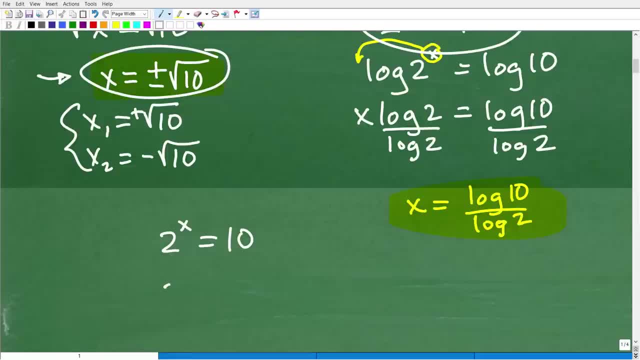 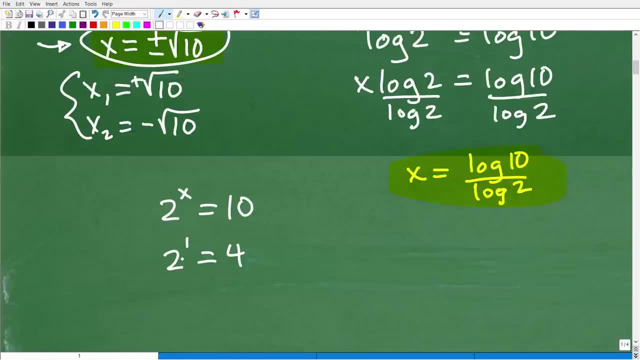 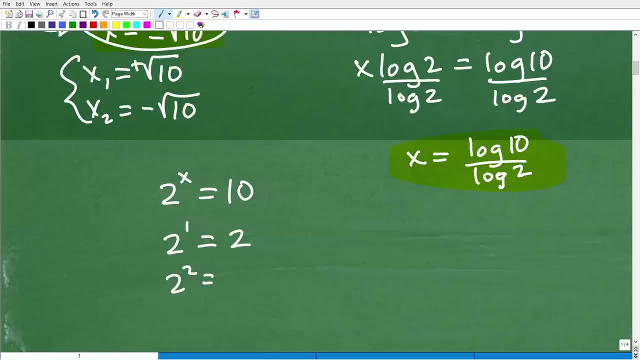 we're like: hmm, two to what power is 10? well, is it 2 to the first? no, because 2 to the first is 4. oh so, let's increase our power. how about two squared? all right, i'm sorry, two to the first is two. excuse me, okay, see, i made a mistake, but i caught myself right. so two to the first is two. 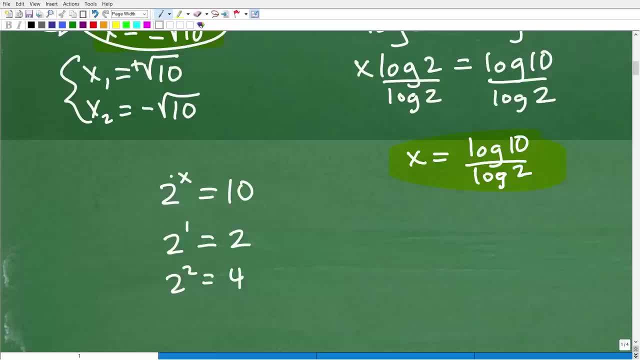 that's not gonna work. two squared is four. okay, i'm looking for two to what power is ten, okay. so i'm just kind of going up here. i'm like: two to the first is two. two squared is four. how about two cubed? well, that's two times two times two, two times two times two, which is of course four. 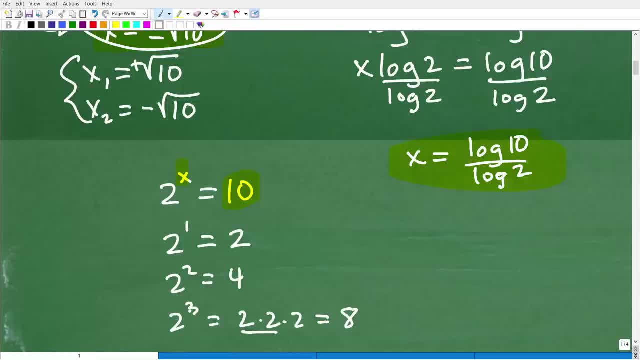 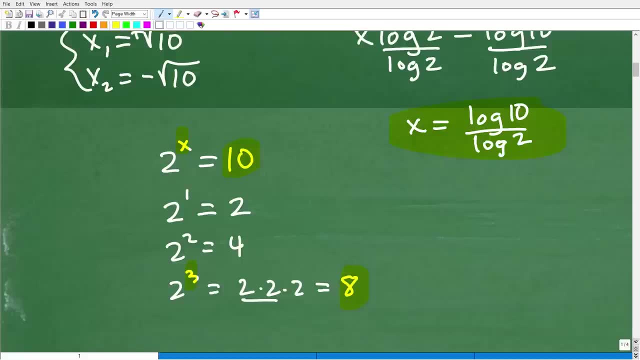 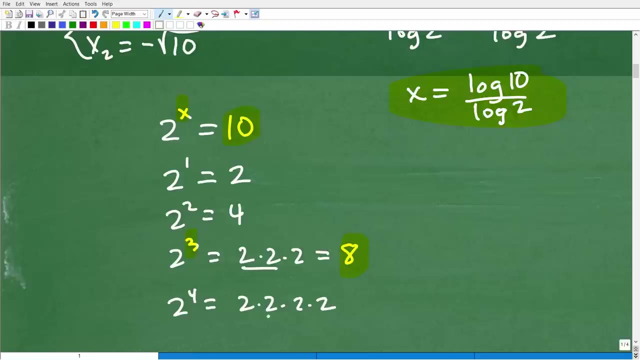 times two, which is eight. so that's pretty close, right? two cubed is eight, uh, so i want ten. so i'm gonna have to increase from three, right, so let's go down here and i go two to the fourth power, which is two times two times two times two. so this is four times four, which is now 16, okay, so 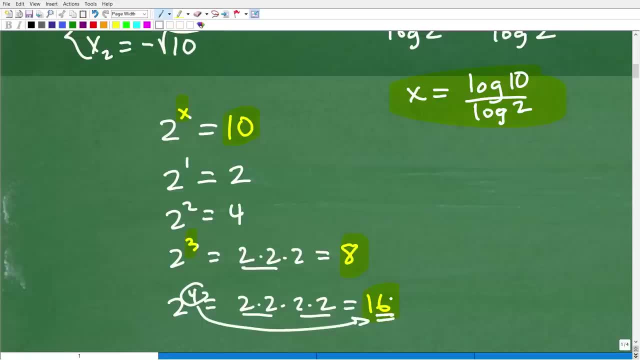 two to the fourth, you know, puts me way over the top. I want 10, I don't want 16. so 2 cubed is a little bit closer to 10. okay. so what does that tell us? well, you can just kind of estimate this. you can be like: oh hey, you use your calculator. 2 to the 3.5, see. 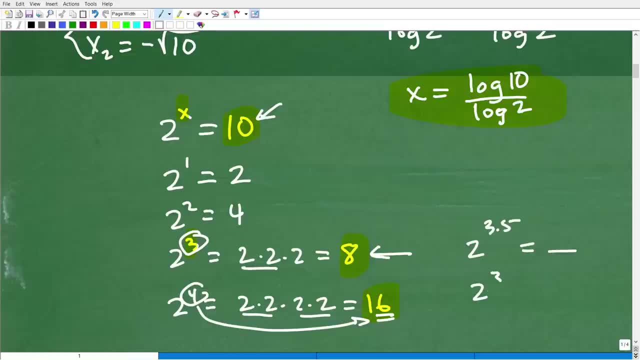 what decimal you get. but your final answer here would be somewhere around 2 to the 3 point, maybe 1 or I don't have my calculator in front of me, but you kind of get the idea. to solve these equations and get the actual, specific, exact answer, you need logarithms. so when you go into your calculator and you